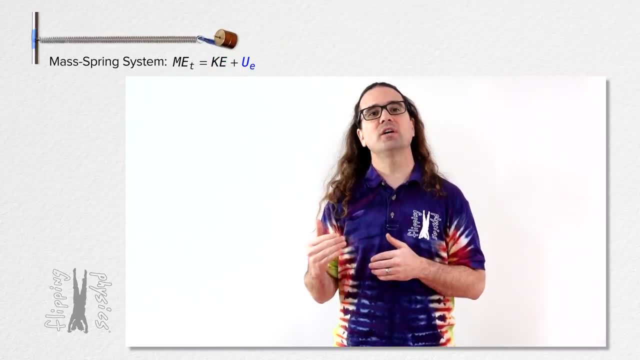 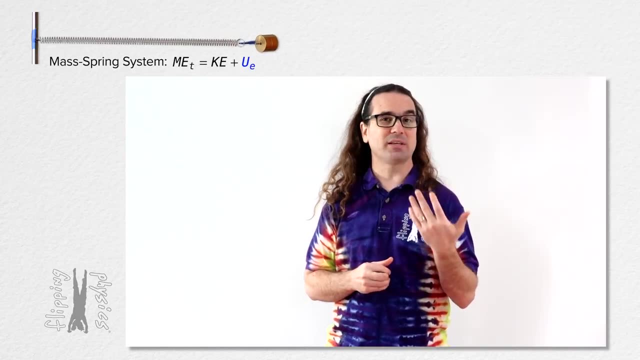 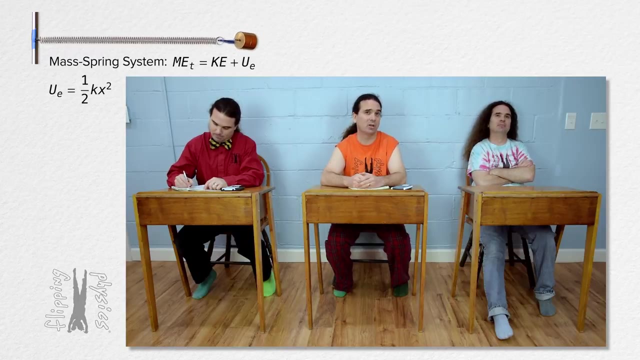 potential energy in the spring. Let's start with just the elastic potential energy stored in the spring. Bobby, what is the equation for elastic potential energy? Flipping Physics. Elastic Potential Energy equals one half the spring constant times, the square of x, the displacement from equilibrium position. 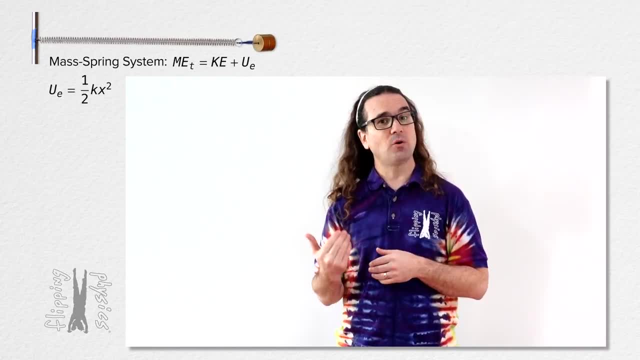 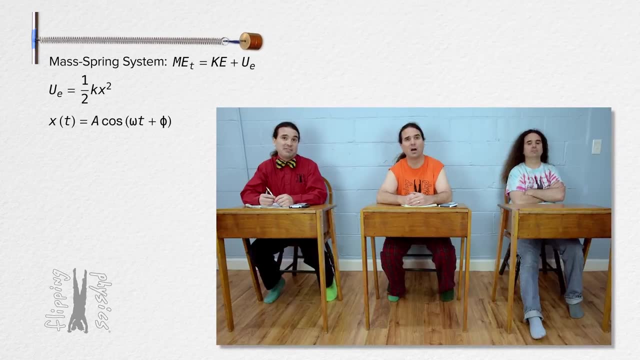 Thank you, Bobby. Billy, what is an equation we derived for the x-position of a mass spring system as a function of time? Position as a function of time equals: amplitude times, the cosine of the quantity, angular frequency times, time plus phi, the base constant. 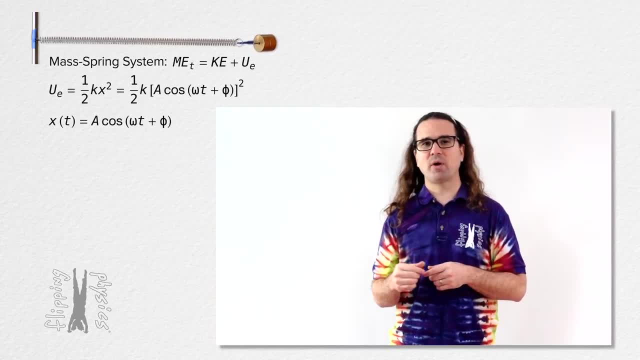 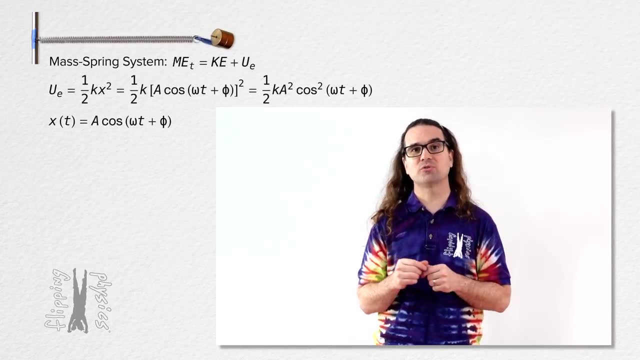 Thank you, Billy. When we substitute that position equation into the elastic potential energy equation, we get one half times the spring constant times amplitude squared times the square of the cosine of the quantity angular frequency times time plus the phase constant Bo. what is an equation for the velocity of this mass which is moving in simple, harmonic motion? 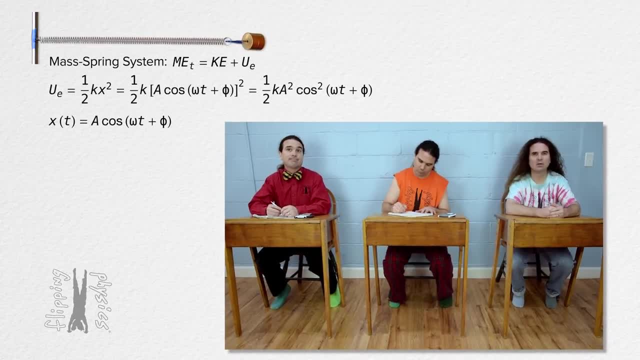 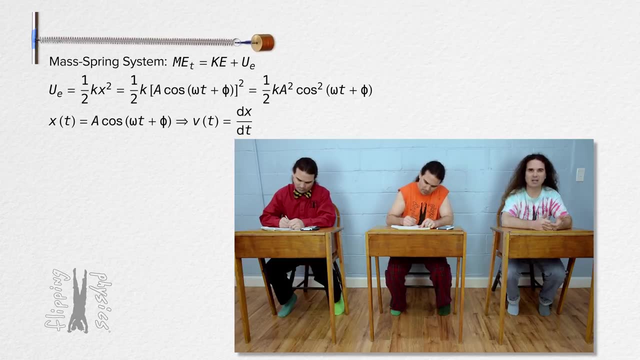 and the equation for its kinetic energy. Take the derivative …. Fine, … with respect to the time of the position equation Billy gave us to get: velocity as a function of time equals the negative of amplitude times, angular frequency times, the sine of the quantity, angular frequency times, time plus the phase constant. 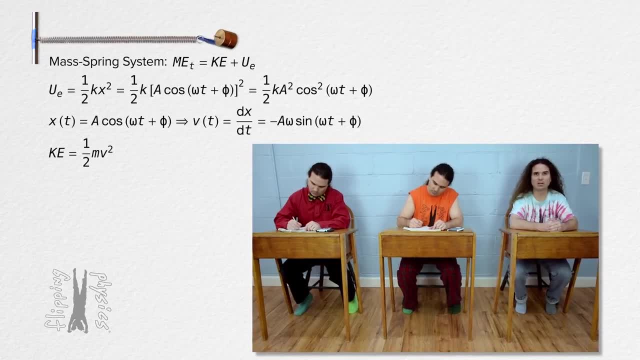 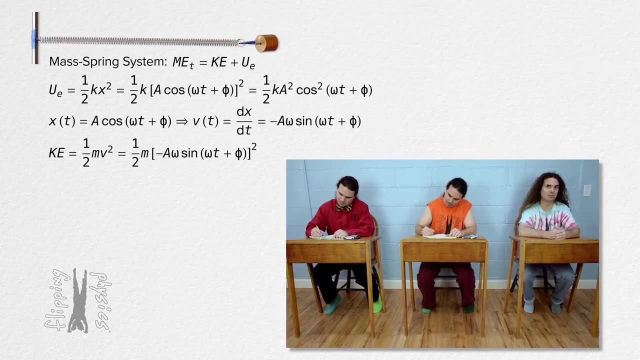 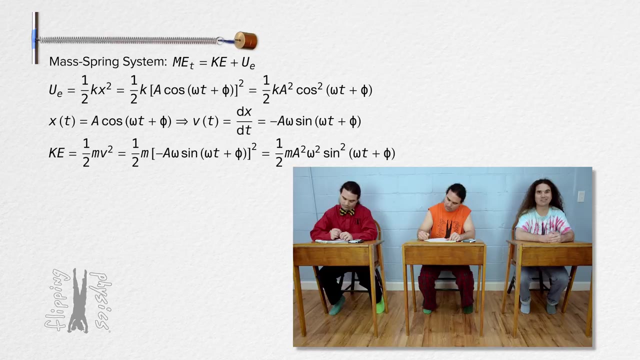 Kinetic energy equals one half mass times velocity squared. We can substitute the equation for velocity into the kinetic energy equation and we get the kinetic energy equals one half mass times amplitude squared times angular frequency squared times the square of the sine of the angular quantity, angular frequency times time plus phase constant. Very nice, Bo. thank you Now. 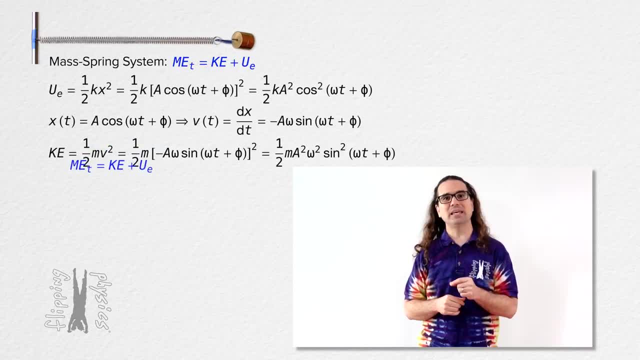 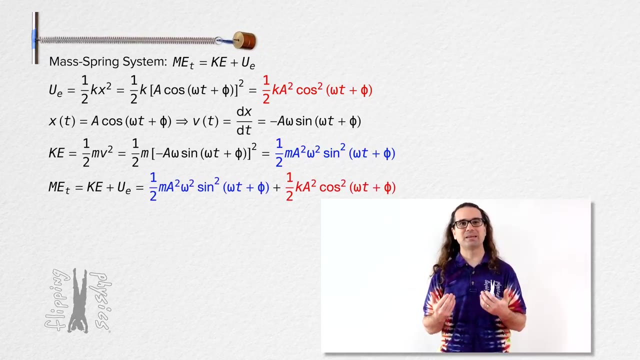 the total mechanical energy of the mass spring system at any point equals the sum of the kinetic and elastic potential energies. We have equations for both of those, which we can substitute in, And we now have an equation for the total mechanical energy of the system at any point. 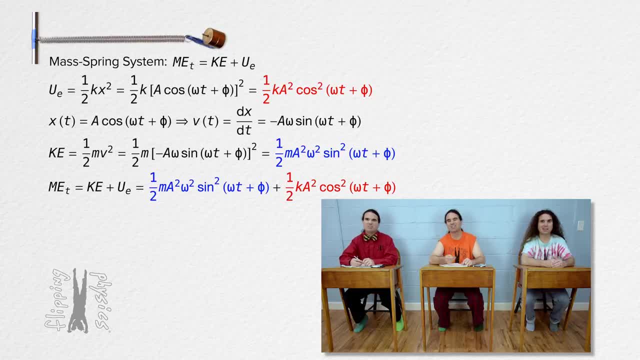 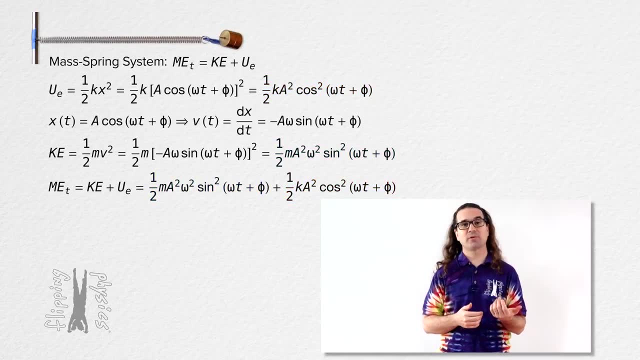 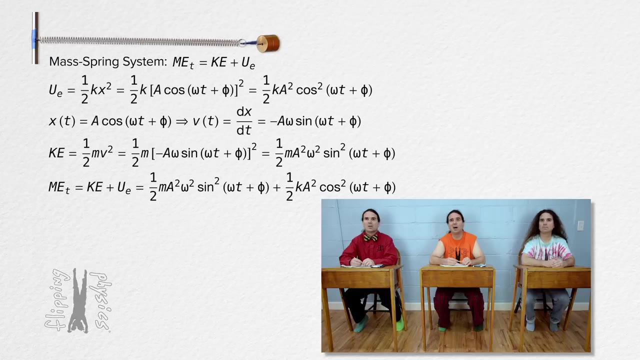 That is just ugly and ungainly. Yeah, It does look confusing. Huh Well, let's simplify it. then, Bo, what is the angular frequency equation for a mass spring system? Uh, I don't know. Just look in your notes from two lectures ago. 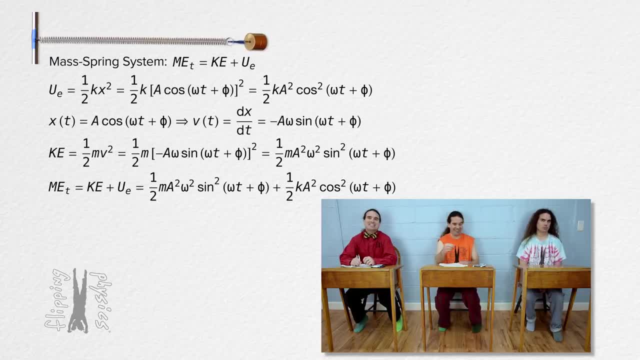 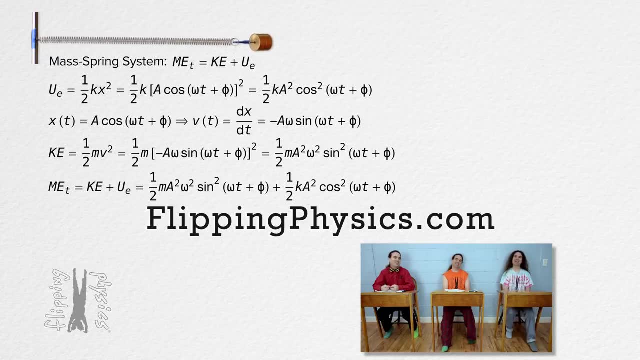 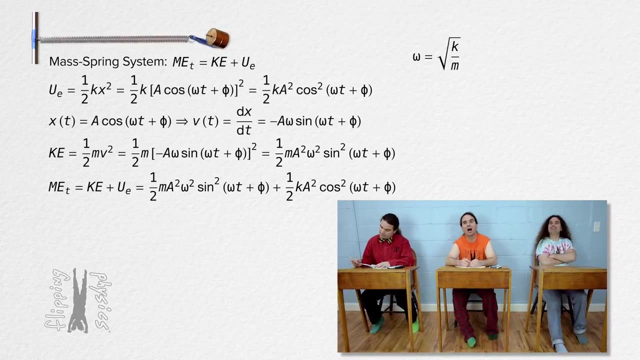 I don't take notes. I just look at the lecture notes you post at FlippingPhysicscom if I forget anything. Nice plug, thanks. Well, yeah, Billy. The angular frequency of a mass spring system equals the square root of the quantity spring. 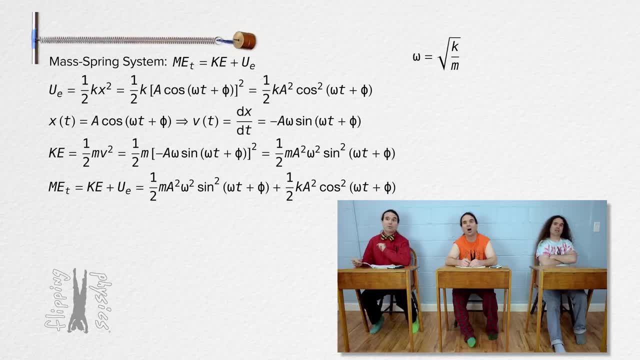 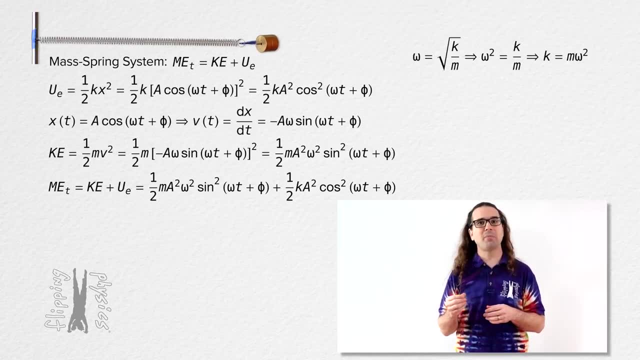 constant divided by mass. Thank you, Billy. Notice then that we can square that whole equation and multiply through by mass to get spring constant equals mass times angular frequency squared. And mass times angular frequency squared is in the total mechanical energy equation for the mass spring system. 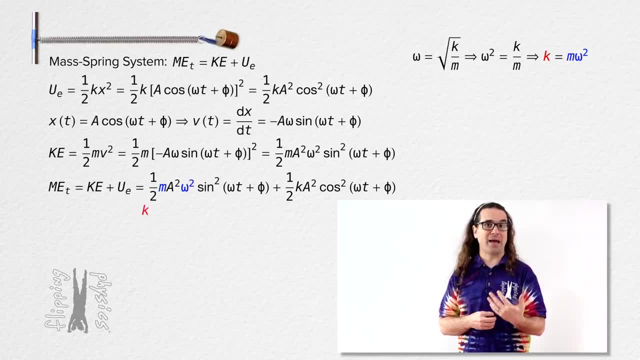 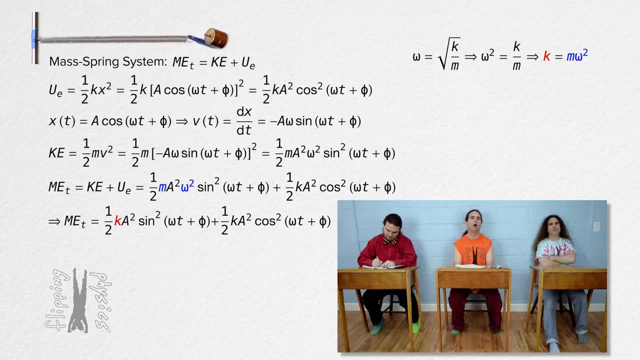 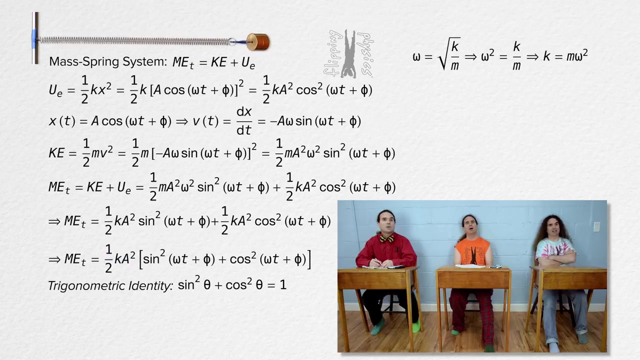 Which means we can substitute spring constant in for mass times, angular frequency squared. Anybody see anything we can do with that equation …. We can factor out one half spring constant times, amplitude squared, but I don't see how that helps …. We can use a trigonometric identity: Sine squared theta plus cosine squared theta equals. 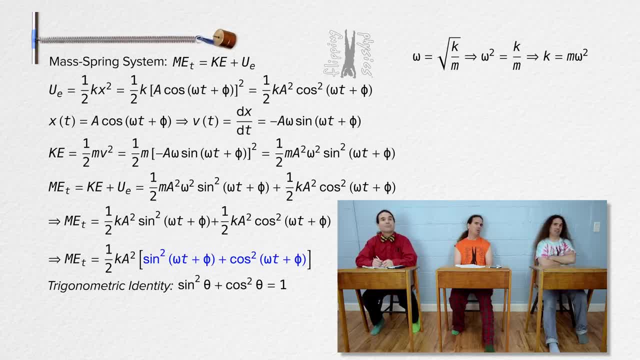 1. … Everything between the brackets equals one. That means the total mechanical energy of the mass spring system at any point equals one-half times spring constant times amplitude squared. That actually makes sense When the mass is at the amplitude or the maximum distance from equilibrium. the mass is at 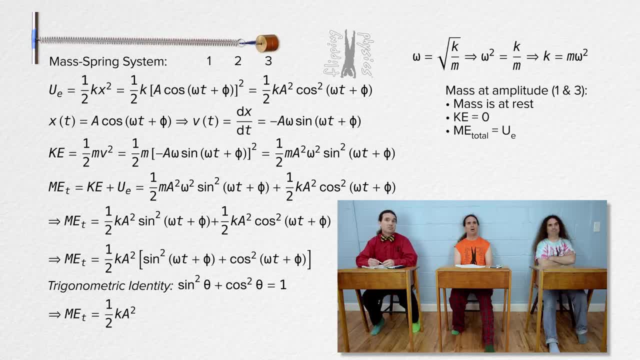 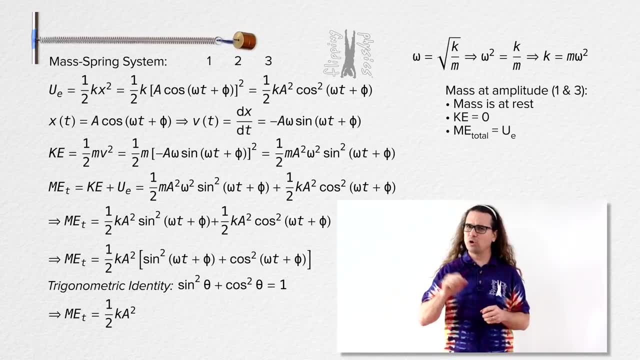 rest and has zero kinetic energy. so all of the mechanical energy is stored in elastic potential energy in the spring. Cool Sure, Very nice y'all. Now. the total mechanical energy of a horizontal mass spring system can also be expressed in terms of kinetic energy when the mass is located at the equilibrium position. 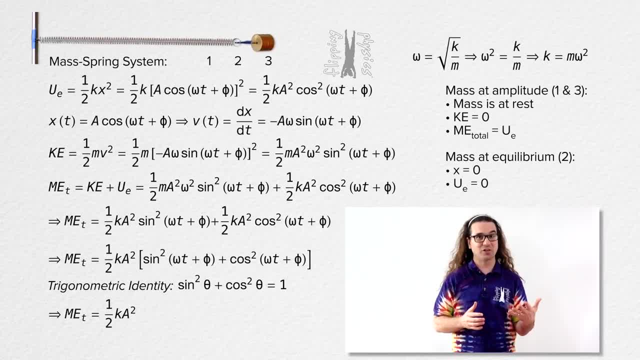 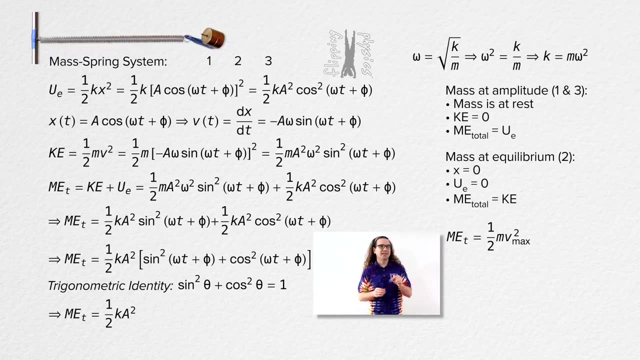 Because the mass spring system has zero elastic potential energy at this location. all the mechanical energy when the mass is at the equilibrium position is kinetic energy. In other words, the total mechanical energy of the system also equals one-half mass times maximum velocity squared. 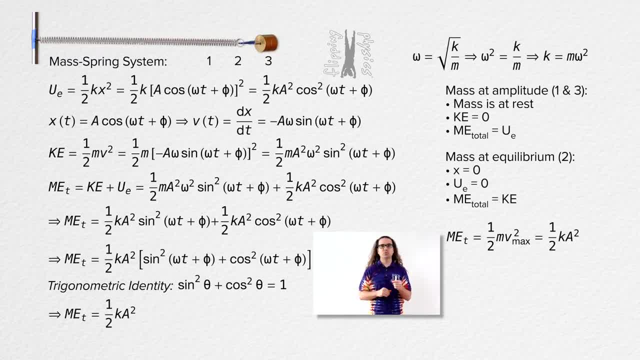 We can set those two total mechanical energies equal to one another, multiply through by two, divide by mass and take the square root of the whole equation to get The maximum velocity of the mass spring system equals amplitude times the square root of the quantity spring constant divided by mass.